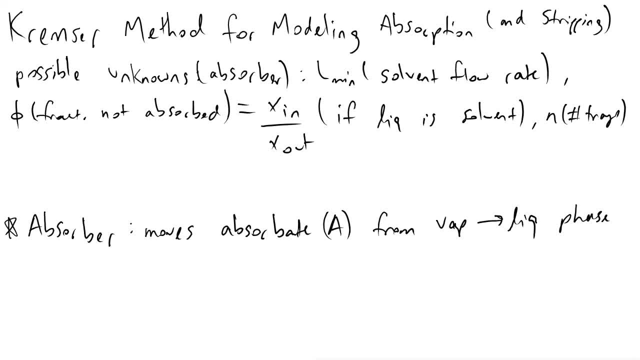 and when working with absorbers, it will be the liquid phase as well as the fraction non-absorbed. And the second variable we define as Φ- and Φ- will be equivalent to x in over, x out. so X denotes the molar ratio of the inlet solvent. so x in And an x out is the molar. 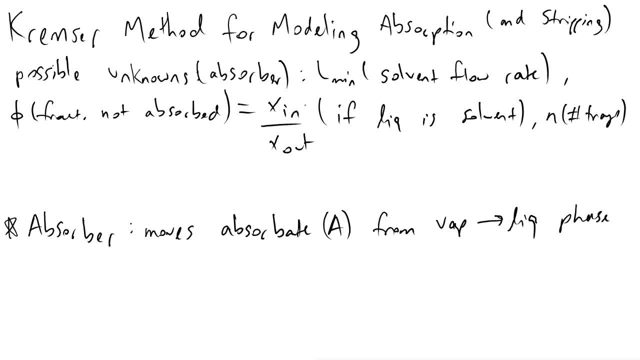 ratio of the absorbate exiting our absorber. And then another variable we will typically have is called little n, and that tells us the number of trays that will be required. And so, as we imagined, we're going to move on to the next step in the distribution of tanks. 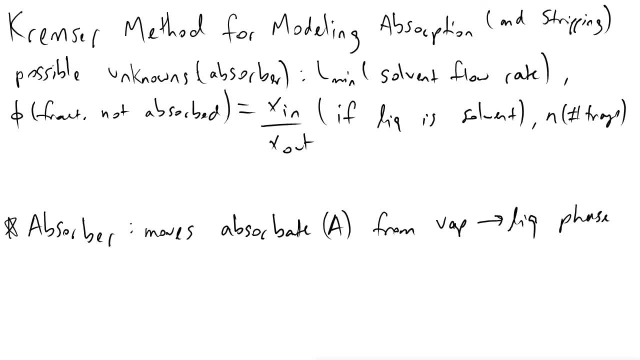 as with many chemical engineering problems, the main issue or challenge is figuring out when is it appropriate to apply this model to a system that we are examining? And the Kremsler method to spell it out is only valid when two conditions are met. The first condition: 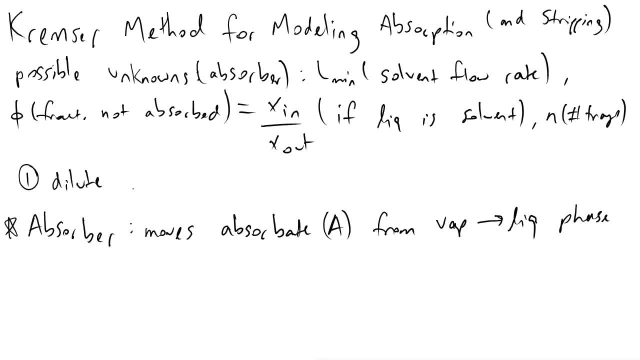 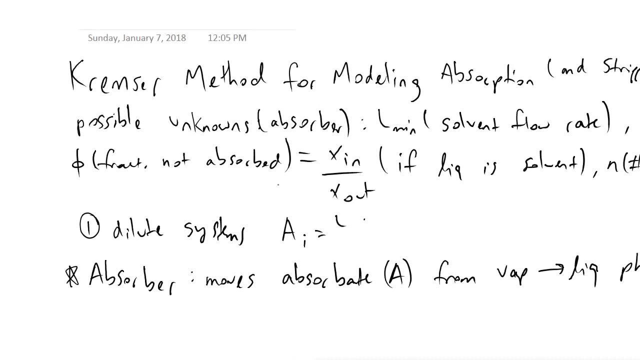 is that we are working with dilute systems, And this is important because it allows us, if our system is dilute, to define something called an absorbing factor and equate that to L-min or L, the liquid solvent flow rate divided by the. 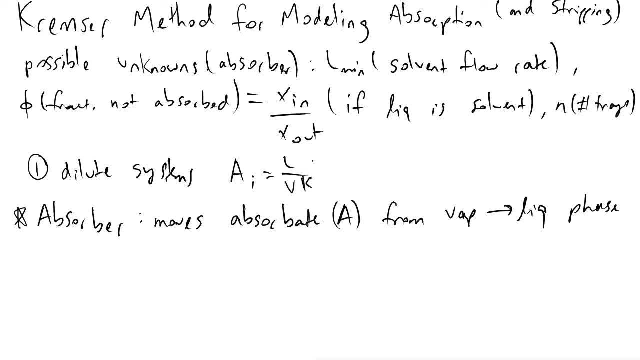 voltage of the liquid solvent flow rate divided by the value of the liquid solvent flow rate, and then the value of the liquid solvent flow rate divided by the value of the liquid solvent flow rate. vapor phase flow rate times the equilibrium constant between the liquid and the vapor phases. 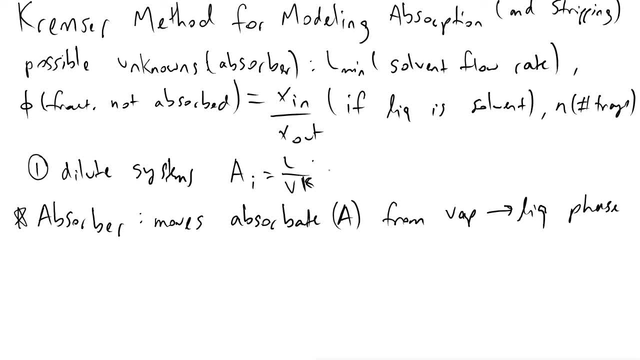 of our absorbate, And if our system is dilute, we can say that this is a constant for all of our trays in our system, And this helps us make a very concise equation that allows us to relate many of these variables to each other, And so to illustrate what's going on here, 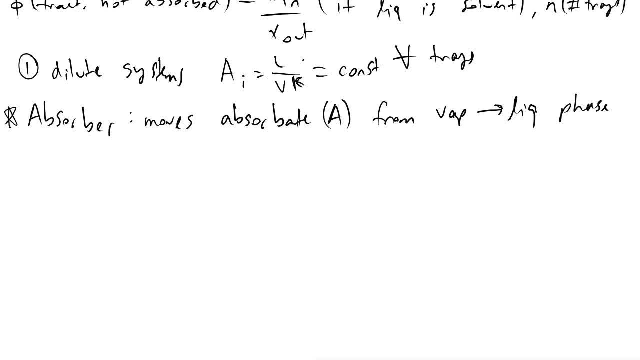 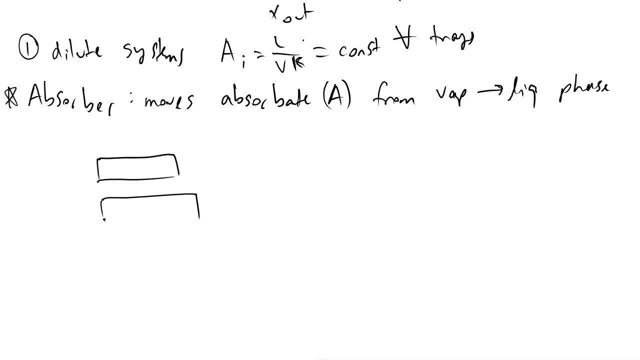 I will draw out how we typically represent absorbers, And what we'll note is that we have trays, So absorber is a composition or collection of trays and a final tray, And the way we number them is like this. So we'll have stage one, stage two, 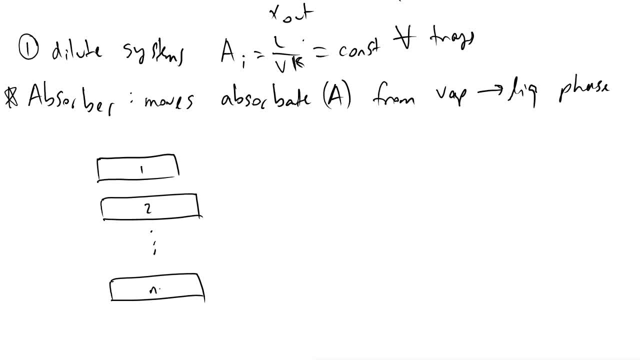 all the way up to stage or tray, And the way we define our flow rates is like this. So we'll have a total liquid molar flow rate denoted L sub zero, And the way this numbering system works is it will be L, so liquid molar. 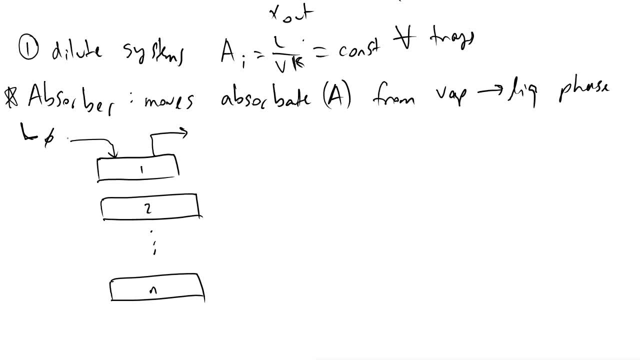 flow rate coming from, whatever stage it's coming from, And so in this case it will be L sub zero, because it's like it's coming from the zeroth stage, And this will have a molar composition of our absorber of x in, and so x n must equal zero for the Kremser method. 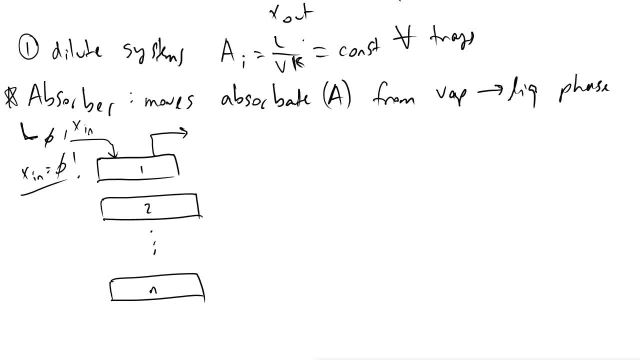 to be applied. And then, leaving tray one, we will have a composition of x one and a liquid molar flow rate L one, And so L one must equal L zero for our Kremser method to be able to to be applied. And then, examining the vapor phase side of stuff, what we have is exiting our top. 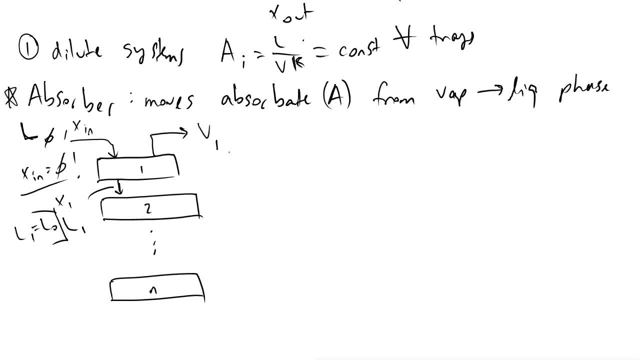 tray a total vapor molar flow rate of V1 with a molar composition Y out. So the molar ratio of your absorbate and your vapor phase exiting our absorber column And the tray right before that will have a composition V2 and Y2.. And so the thing to note here is that with the Kremser method 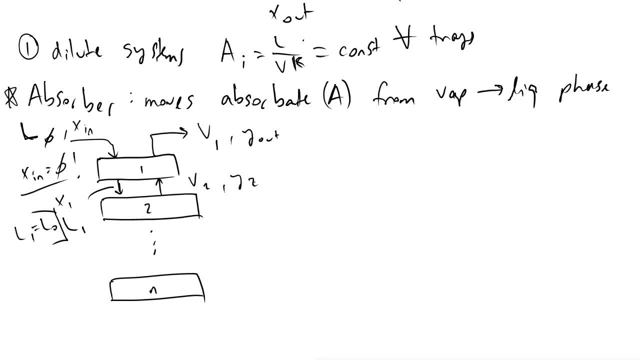 or with any equilibrium relationship. we know that Y out must be in equilibrium with X1. So the streams that are exiting a tray must be at equilibrium, And that is to say that Y out is equal to K, some equilibrium constant times, X2.. I'm sorry, X1. So that is a key. 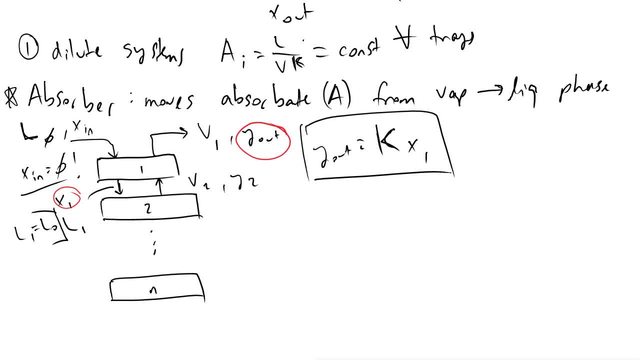 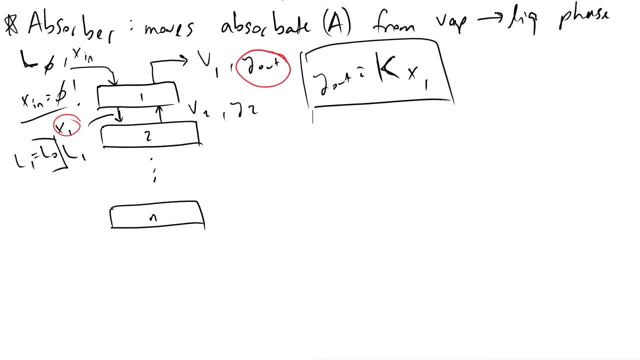 relationship, to understand when working with absorption And to examine what's happening in the bottom tray of our absorber column. we will have the liquid exiting L sub N and that will be a composition of X. out And entering our absorption column we will have a vapor molar. 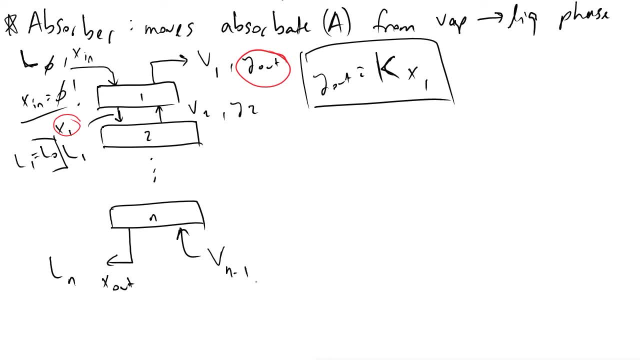 flow rate of V sub N minus 1,, because it's originating from the N minus 1 tray, as well as a composition, Y sub N minus 1,, which is equivalent to Y in. And so the thing to note with absorbers is that we are, because we're moving our absorbate from the vapor to the liquid phase. 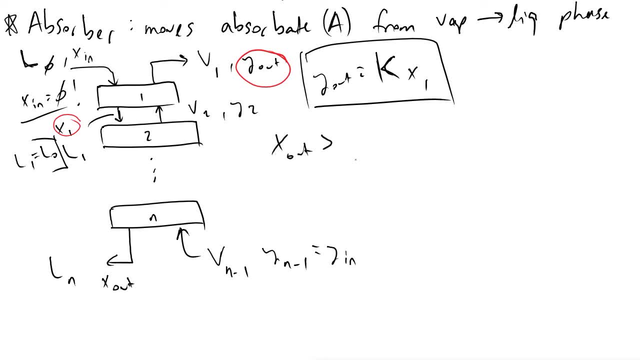 we're not removing gas, And so if we avoid the junction of the vapor and let it simply sink in, X out will be more concentrated, will have a higher molar ratio of your absorbait than X in, And the opposite can be said of the vapor concentration. so Y out will have 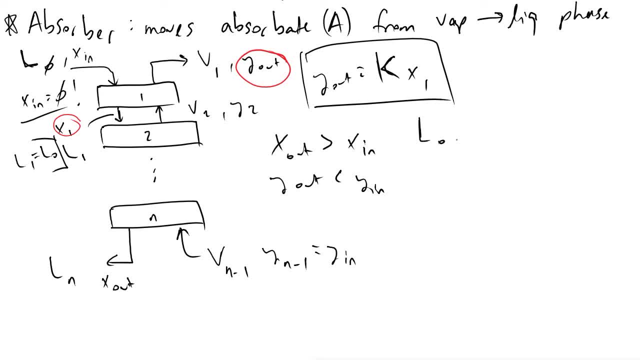 a lower concentration than Y in, And so the reason the Kremser method is able to be applied is because we were able to say that L 0 was equal to L N, And so I suppose at any point in a re problems we will actually 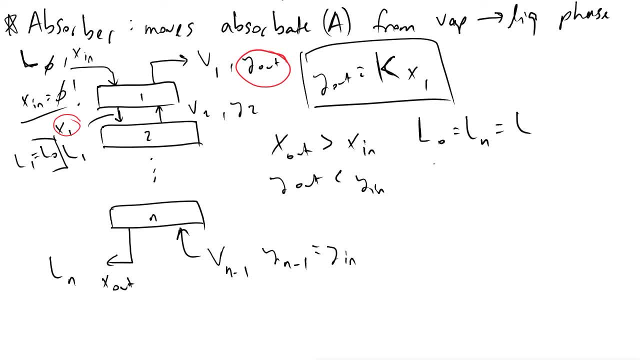 we can let that equal some constant L, and then we can also say that the same can be said for the vapor flow rate. so V1 would be equal to V, sorry, Vn minus 1, which we can just let that be equal to V. and now what we can do is define an absorption factor. I will call it Ai and that: 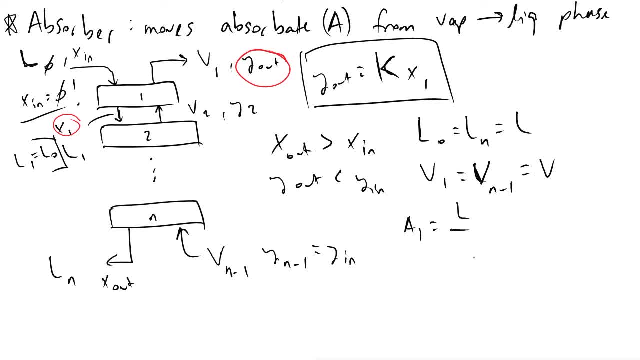 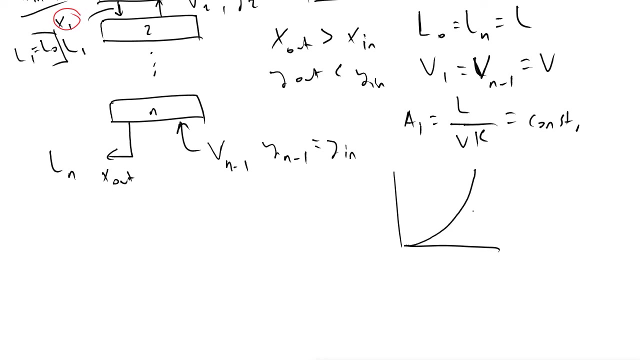 will be equivalent to L over V times K and this is equal to a constant value. and the reason we can say it's constant is because we've already noted that L and V are constants because we work in a dilute regime. typically, equilibrium curves at higher concentrations will look like this: 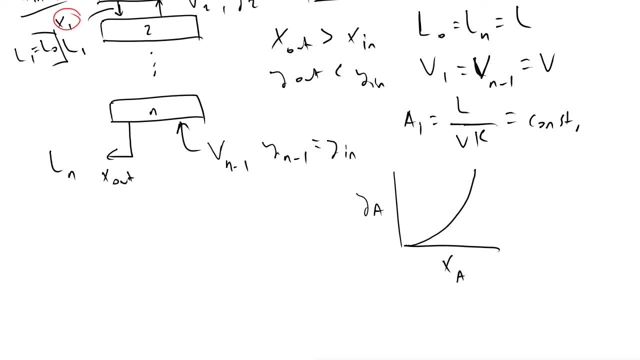 but if you notice how initially we can approximate this nonlinear function as linear if we're working in dilute areas, we can say that if we zoom in here it's linear or it's approximately linear enough that we can apply these kinds of math equations to these models. and just to clarify so in this: 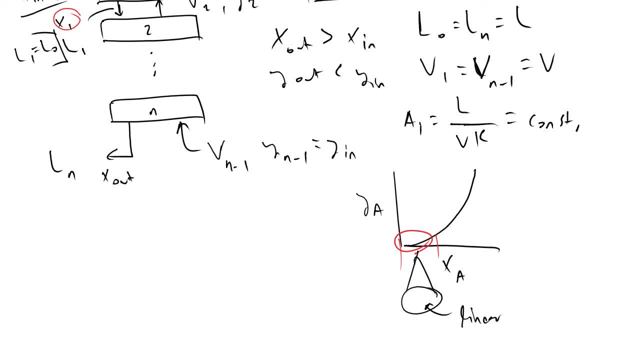 regime when we have the linear slope. initially, what this allows us to do is also let K equal a constant value at low concentrations, dilute okay. and so to get to the main point here, the Kremser equation tells us that the fraction not absorbed V is equal to a minus 1 divided by a to the n plus 1 minus 1. so this is the main takeaway from. 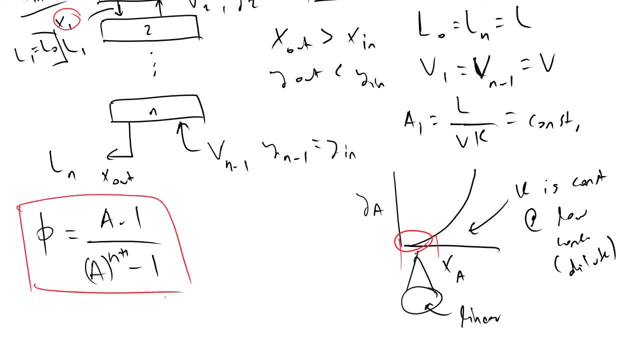 the Kremser equation, and n is the number of trays and a is the absorption factor. I'm sorry, I should write a sub i here, a sub i. and the difference between n and V. the DON certainly does matter. now, all about n and V here, what it. 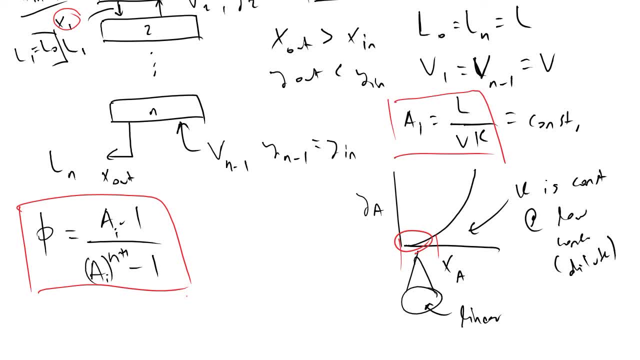 actually stands against. lets us always take advantage of this term where we are salating between an expected fraction of x and an expected fraction of Z. the equation that theanca put together is the least important thing. it always looks the same. it looks the same, the same thing. so let's still have a small margin of S cost. x is good. 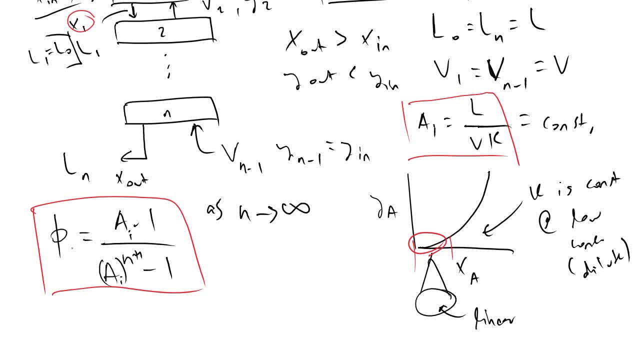 gets very large and phi, the fraction not absorbed goes to zero And, as a sub, i goes to infinity. so as we increase our absorption factor, as we increase the so a is proportional to our solvent flow rate for an absorber, which is l. So as we flow more and more solvent through our